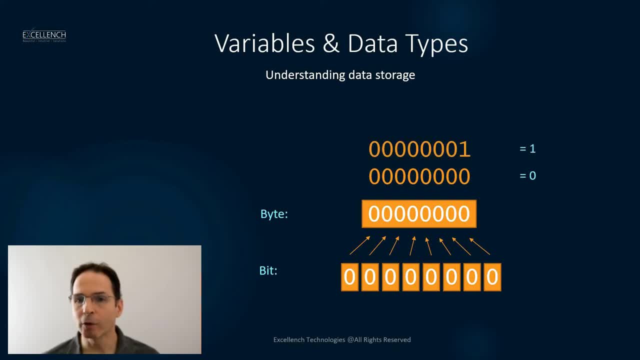 zero. If we turn on only one bit on the rightmost bits, we define that to represent the number one. If we turn on just the second bit from the right, we define that byte to represent the number two. Are you thinking about the number three? Do you have any guess? 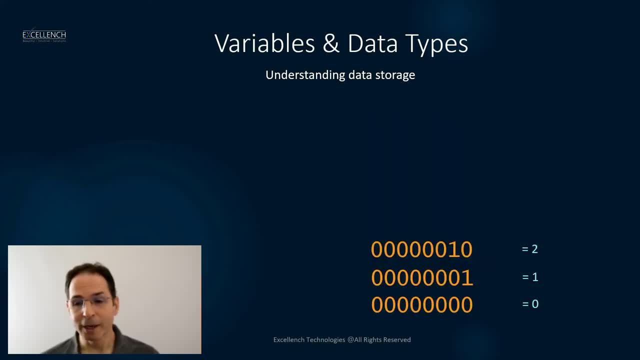 Well, we already know how we define zero, one and two to be represented by bytes. Let's see. Let's see how this has been defined. actually, We assign each bit a number. The rightmost bit is assigned the number one. The second bit from the right is assigned the number. 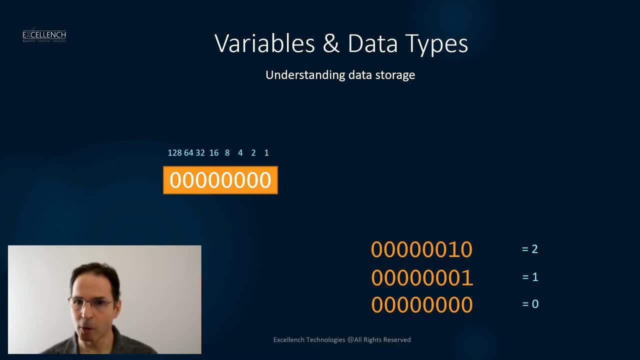 two, The third bit is assigned the number four, and so on and so forth. You can see there is a pattern here. One multiplied by two is two, Two multiplied by two is four, Four multiplied by two is eight, et cetera, et cetera. Actually, since each bit has only 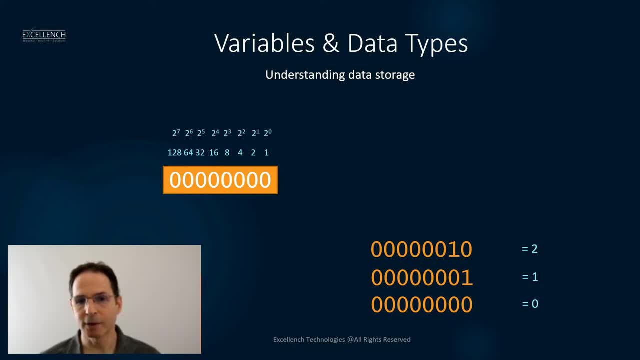 two options. this pattern is received by taking the power of two. So two to the power of zero gives us one. Two to the power of one gives us two. Two to the power of three gives us four. Two to the power of two gives us four, et cetera, et cetera. We can say that up to 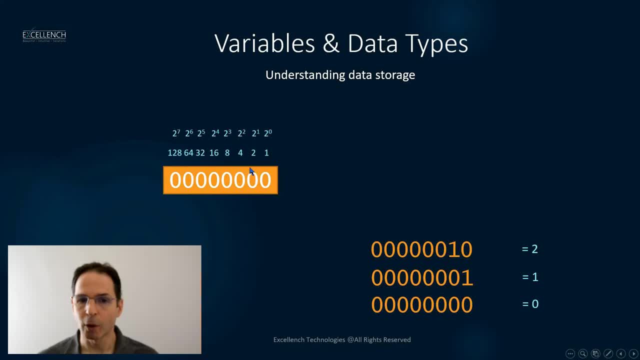 the third position. if we only look to the right, at the two first bits, we have up to two by two possible combinations of these two bytes. These two can either be both turned off, can either be turned on, or can either be turned off or can either be turned on. 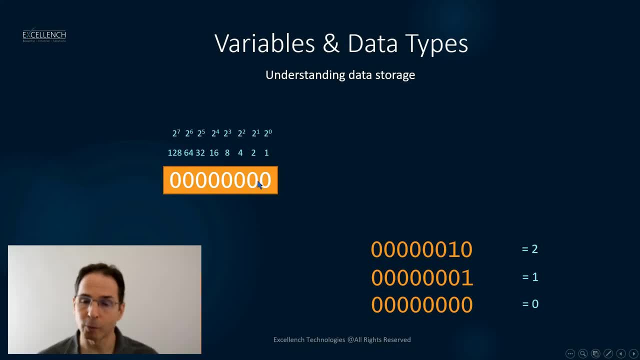 and either one can be turned on while the other is off. We therefore have four possible combinations, and that's why the third bit is represented by the number four. If we take the three bits, how many combinations do we have for three bits now? Well, it turns out. 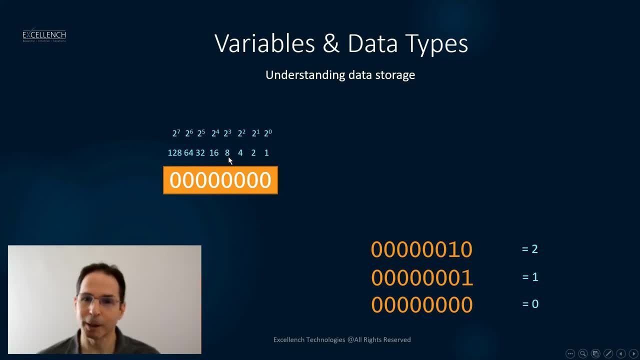 we have eight possible combinations. Take a sheet of paper and try it out. These are the rules. that defines our pattern for representing numbers within a byte. So, if we follow this rule, the number three is now represented by turning on bit number one and bit number two. Bit number one represents the number one. Bit number two represents 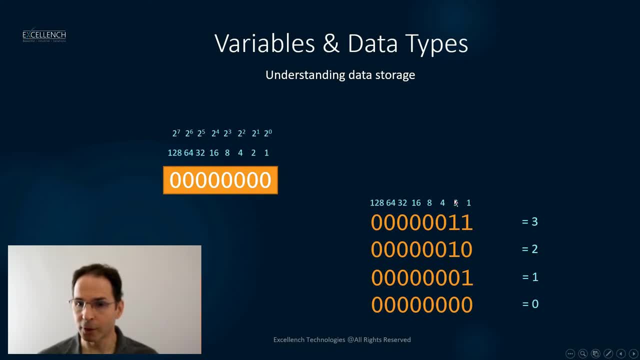 the number two. We added those two together and we get a three. The number four will be represented by turning on the third bit, because number four is representing the third bit. Using this same logic, how do we represent the number twenty six? We? 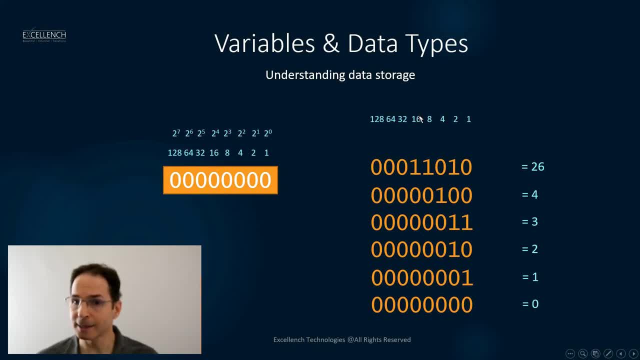 turn on the bit that is represented by sixteen. Then we turn on the bit that is represented by the number eight. 16 plus 8 that gives us 24. so we're missing two. we have the second bit that is represented by the number two to add on to that. so these three specific bits. 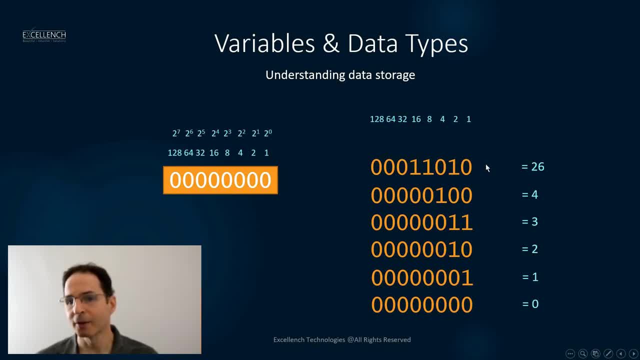 come together to revisit to represent the number 26. now, if we turn all eight bits, what do we get? we need to add 1 plus 2 plus 4 plus 8 plus 16 plus 32 plus 64 plus 128. that brings us to 255, so the largest possible number whole. 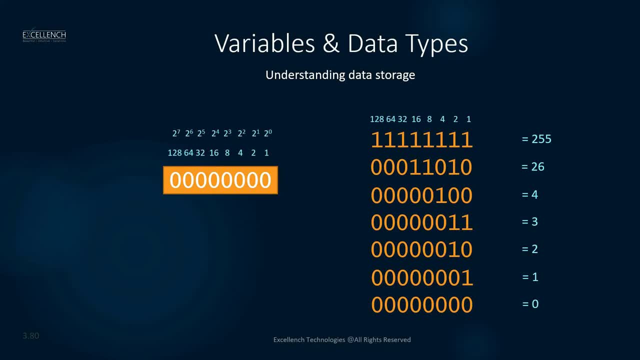 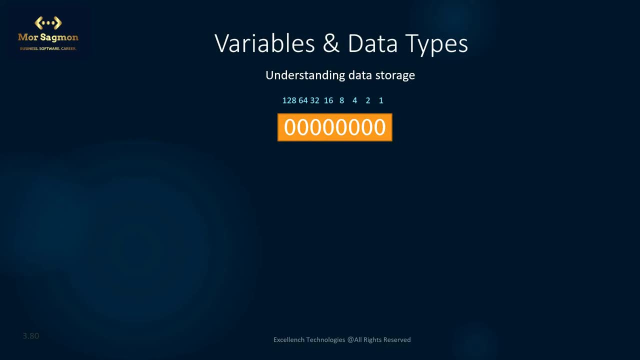 number that we can represent using a single byte is 255. so how do we represent larger numbers? how do we represent 256? how do we represent 2008? well, we do that by concatenating two bytes together. in this way, we have extended the 8 bits. 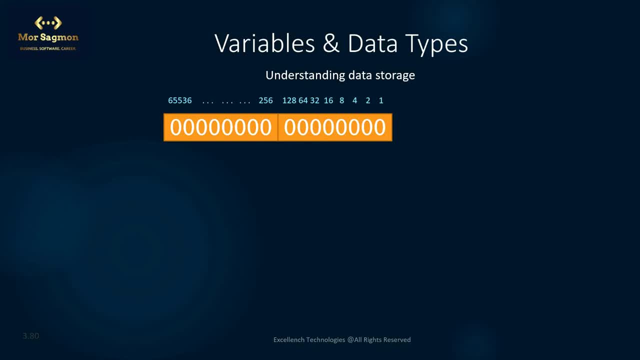 available within one byte into 16 bits. that now allows us a combination of 16 possible ones and zeros along those two bytes, whereas the 16th bit represents a. 16 possible ones and zeros along those two bytes, whereas the 16th bit represents the 65,536. so you can imagine that many combinations are possible with 16 bits. 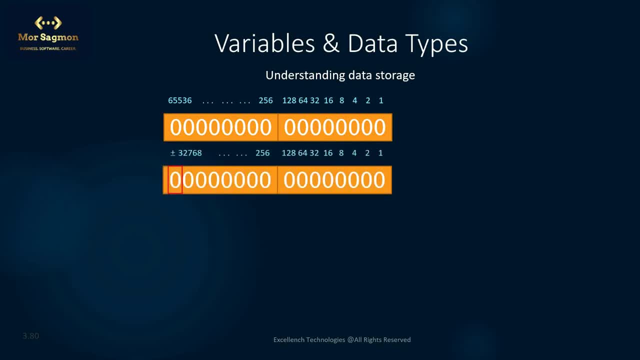 however, we must consider representing also negative numbers. for that we sacrifice the most significant bit, which is the leftmost bit here, to represent the negative sign, in case we are representing signed numbers as opposed to unsigned numbers. so with unsigned numbers we use all of the bits available. 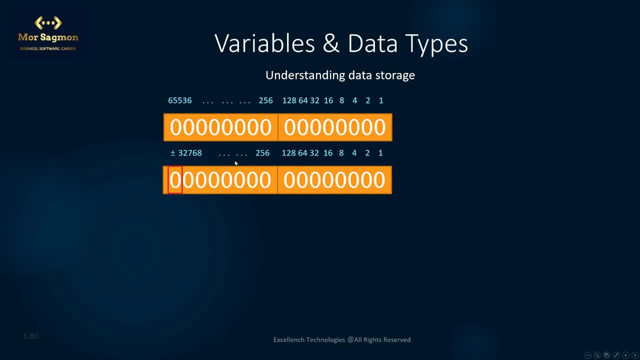 to represent positive numbers only with signed numbers. we represent both negative and positive numbers by using the leftmost or most significant bits along with two complements of the rest of the bits. let me show you what I mean. this is the regular representation of 266. we're taking 256, we're adding 8 and we're 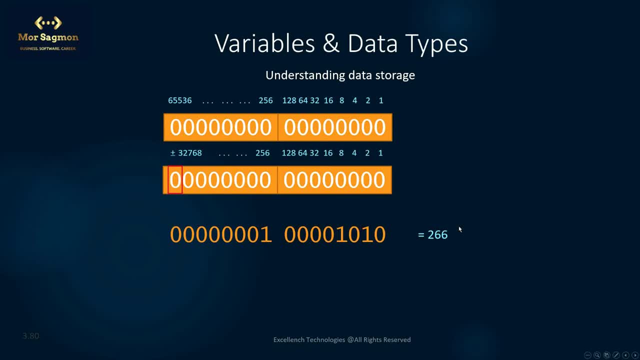 adding 2, that brings us to 266. now, in order to do the trick to represent the negative 266, we first take the 266 representation and apply the first complement to it, which is basically just toggling all of its bits. so every bit that was 0 now becomes 1, and every bit that was 1 now becomes 0. this is 266. 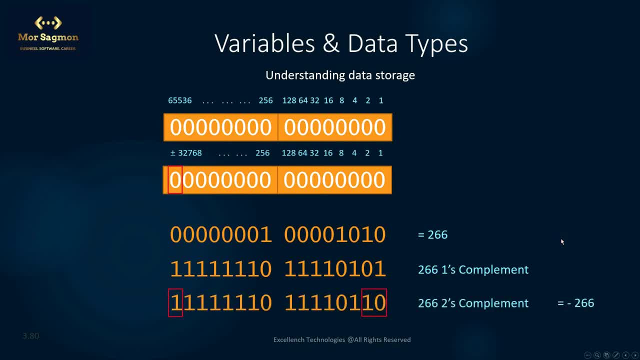 first complements, then we do the second complement on that representation, which is basically adding 1 to the ones complement. adding 1 in binary means that we are running from the right, from the least significant digits, from the right to the left the direction on a representation and whenever we 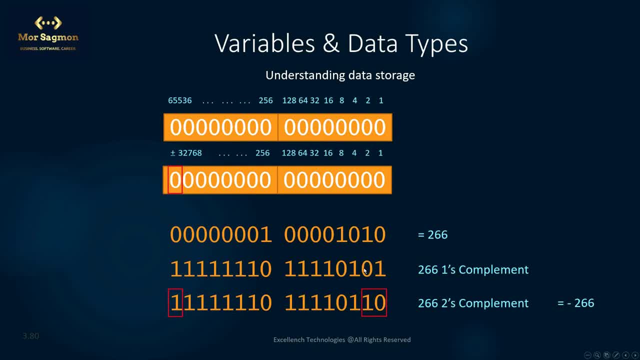 encounter the first zero, we stop and then we flip, we toggle all of the bits that we encountered so far. so in our example, we start with the first bit, which is 1, since it's not 0. we are continuing to the next bit from right to left, which is 0. so now we've 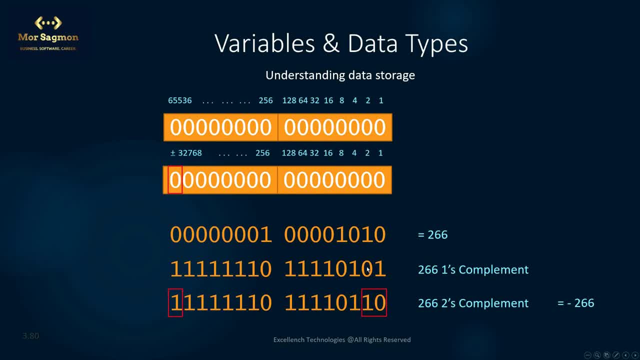 encountered our first 0, so what we do now is that we flip that 0 to 1 and the previous one to 0. so, as you can see, these two bits were flipped back to what they were originally by just adding 1 to the ones complements. 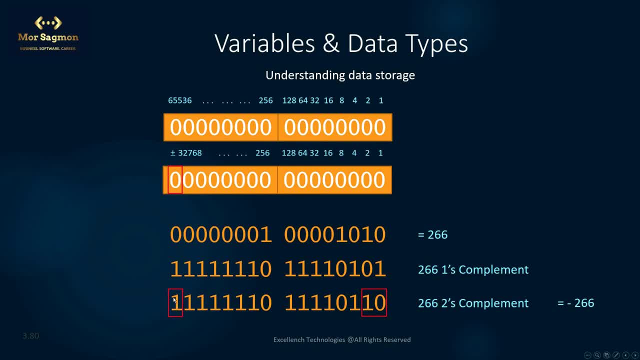 and our leftmost bit is turned on, which tells us that this represents a negative number. so this way we tell our computer that this is the negative number, in case we have defined for the compiler that this is the signed number. so this bit is used to represent the negative number, if it is one, and that it must be. 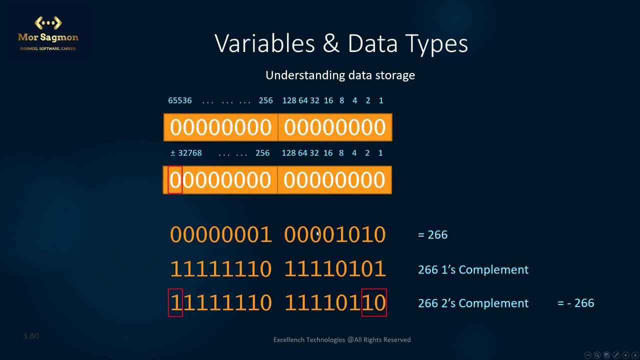 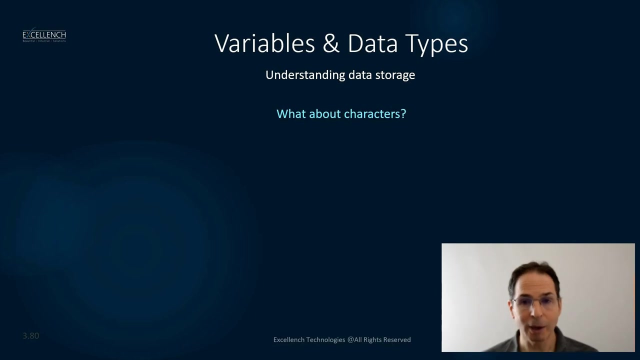 de-complemented back to this representation of 266, together with the minus sign that is represented by this bit. So this is how we would represent minus 266.. So we know how we can represent numbers. How about characters, strings? What we can do is decide that each character is represented by a numeric code. 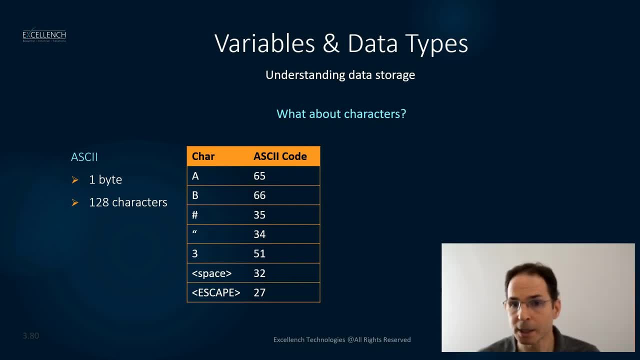 Now, since we already know how to represent and store numbers, we can store strings by storing many, many numbers, one after the other. For that we have an ASCII table A-S-C-I-I. That is the very first table that was defined in the first days of computers. 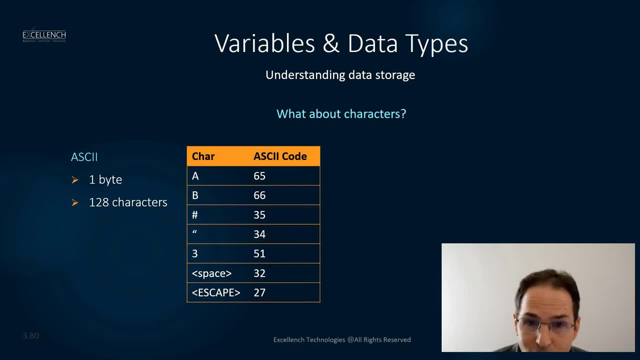 to represent the alphabetical set of strings of characters. Now, an ASCII table has only one byte to represent characters, And we know that one byte is very limiting. We can store up to 255 numbers or 128 characters if we omit the leftmost bits. 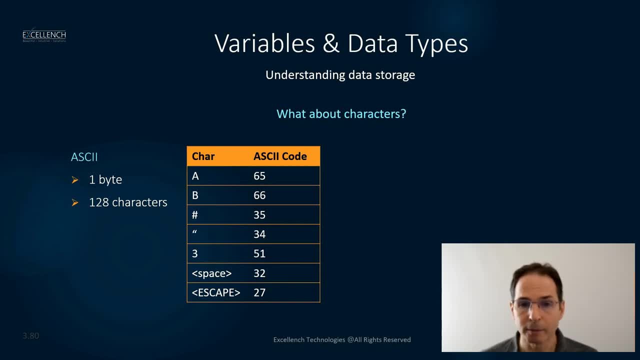 But the ASCII table is still very popular and it represents all of the characters in the English alphabet and string. But there are going to be some other characters as well. For example, the letter A in capital is represented by the number 65.. 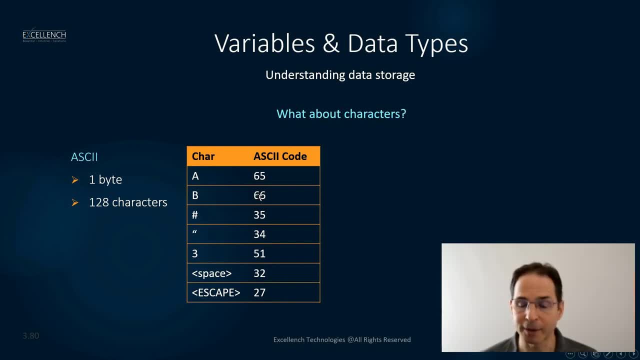 The letter B in Capital is represented by the number 66.. The space-character is represented by 32.. The double quote is represented by 34.. The number 3 as a string-as-a- character- not as-a-number- is represented by 64..